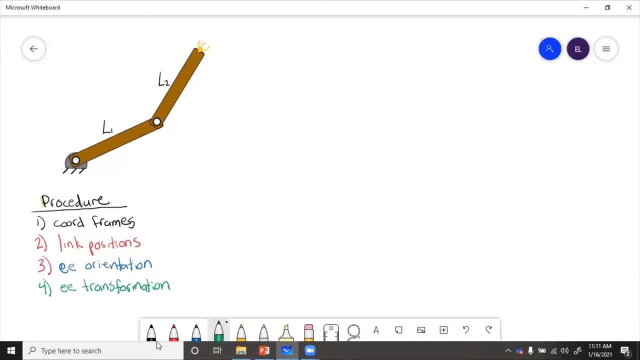 What angle is the end-effector pointed at? So what angle is the end-effector pointed at? We'll say: for all of these, this is a planar manipulator. So we'll say: z comes out of the page because z is the rotation axis. 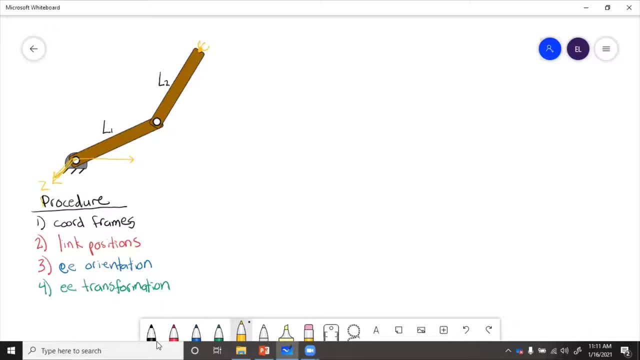 And then for the base frame we have x- zero to the side and y- zero points up. So we'll say z comes out of the page because z is the rotation axis. Then each next frame is on the link that follows it. 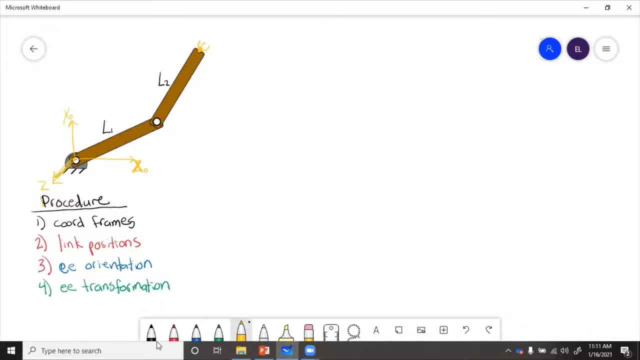 So here we know that x1 has to point along that link And then y1 is perpendicular. And then, finally, for the end-effector, x2 points along that link and y2 is perpendicular. So the angles that these rotate, So the angles that these rotate. 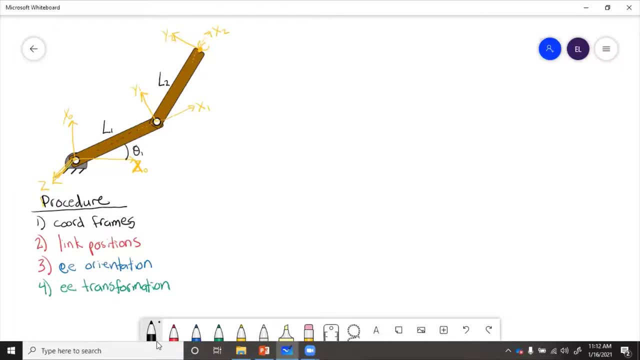 This is theta 1 between frames 0 and 1, and then theta 2 between frames 1 and frame 2.. So step 2 is link positions. So where is the origin of frame 1? We want to give that in the 0 frame. 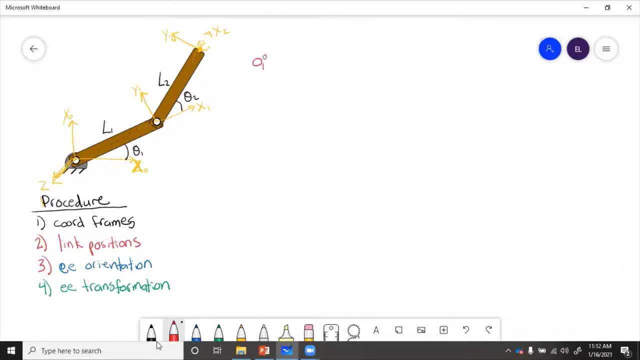 So origin of frame 1 with respect to frame 0 is going to be the x and y positions. So to get here, from here we go to the side and up, So that's going to be in the x direction. we have l1 times cosine of theta 1,. 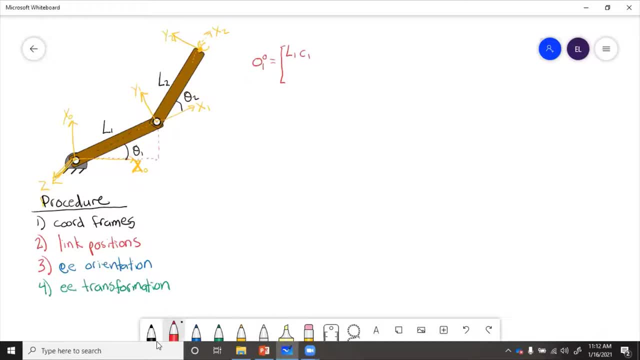 and then l1 times sine of theta 1 in the y, And then for the second origin, origin of frame 2 with respect to frame 0, we have to get from 0 to 1 to 2.. So in the x direction, to get from 0 to 1, we had l1 cosine theta 1.. 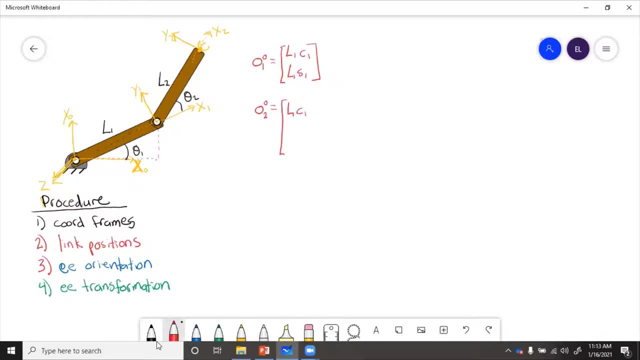 And then to get from 1 to 2, we'll have l2, and it's going to be times cosine, not just theta 2, but also we have to add theta 1, because, remember, we're giving this relative to the base frame. 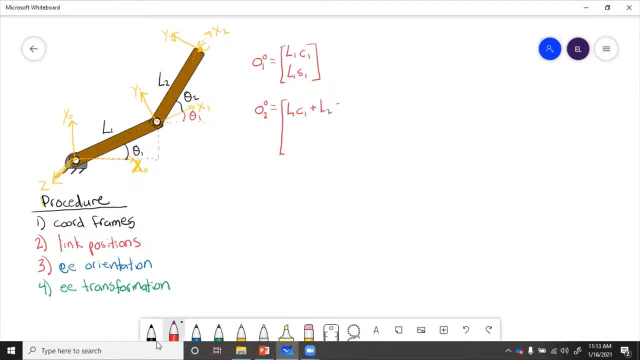 So plus l2 cosine of theta 1 plus theta 2. We abbreviate that as c12.. Then similarly in the y direction we'll have l1 sine of theta 1 plus theta 2.. Then, similarly in the y direction, we'll have l1 sine of theta 1 plus theta 2.. 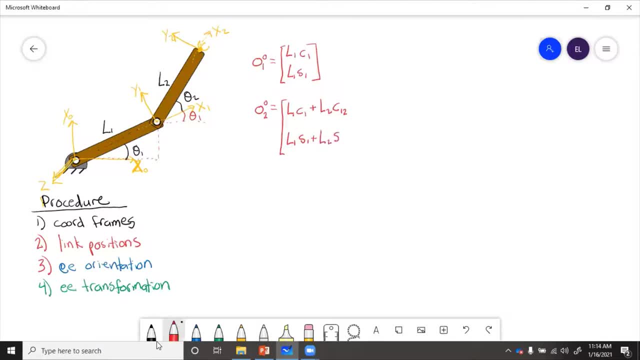 Then, similarly in the y direction, we'll have l1 sine of theta 1 plus theta 2.. And then, finally, we need end-effector orientation. So that is, what angle is the end-effector rotated? at r of 2 in frame 0 is going to equal the rotation matrix. 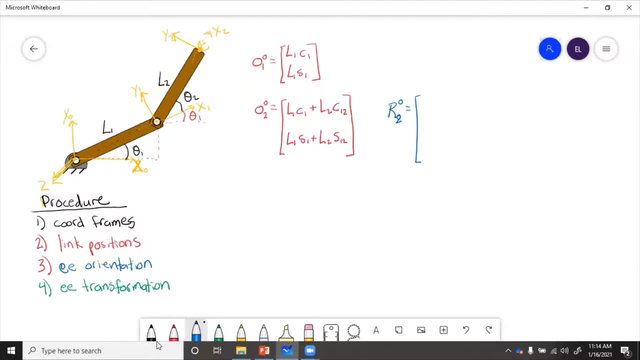 of that angle that it's rotated. So this is going to be r around the z, theta 1 plus theta 2.. So we have c12, s12, minus s12, c12, 0, 0, 0, 0, 1.. 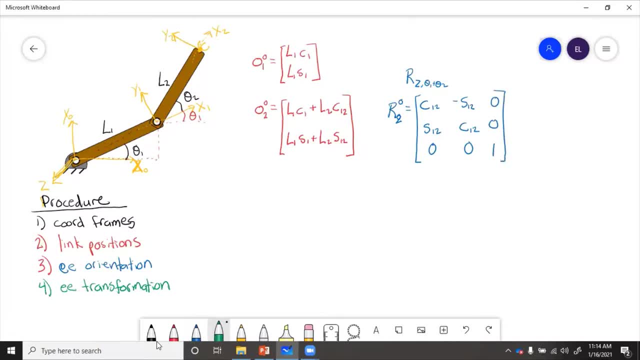 And then the transformation t2, frame 0, equals the rotation r20, the position: 0, 2, 0, 0, 1.. Remember, this is the zero vector, so it's actually three zeros. 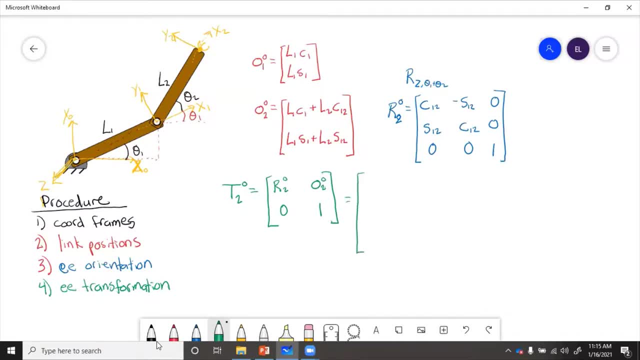 So if we put all those parameters in, then we have c12, s12, 0, minus s12, c12, 0, 0, 0, 1.. That gives us the orientation, And then we need the position. 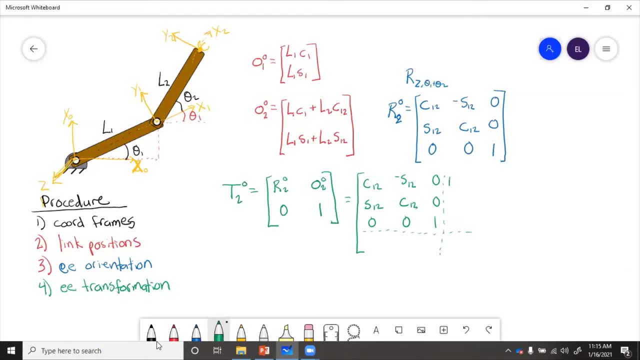 So this 0, 2, 0 is l1, c1, plus c2, 0, 0, 0, 0, 1.. So that gives us the orientation, And then we need the position. So this: 0, 2, 0, plus l2, c12, l1, s1, plus l2, s12, 0.. 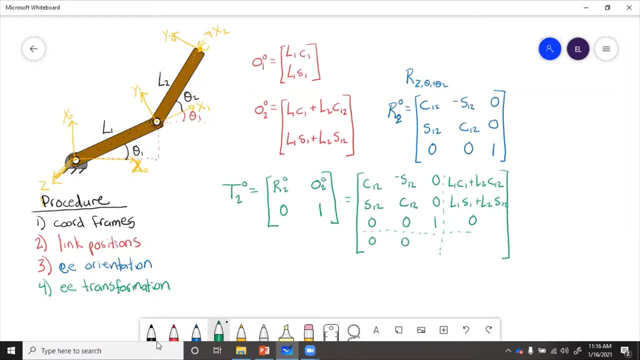 And then remember to make this square matrix. we put 0, 0,, 0 in the orientation and 1 in the position. So this is the transformation matrix to get from the base here to the tip here. So now let's put some numbers in. 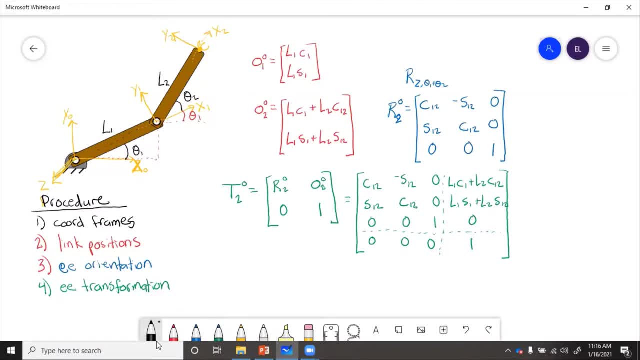 Let's say, if we're given l1 equals 0.1 meters, l2 equals 0.2 meters and theta1 equals theta2 equals 30 degrees, find the position of the end effector. So the pose of the call will have position plus orientation. 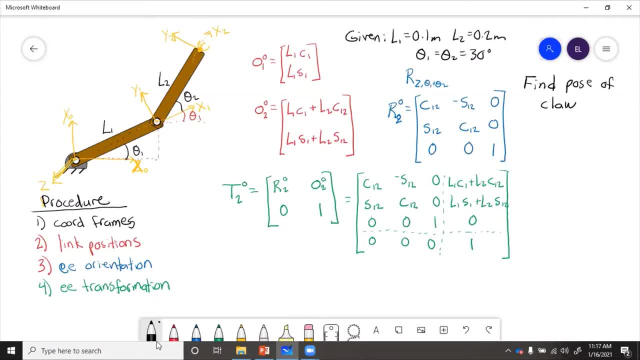 Now the position will come from this column, And that's something that no doubt you have calculated before in physics, dynamics, kinematics, so on. The orientation is a little bit new, But all we have to do here is put in the numbers. 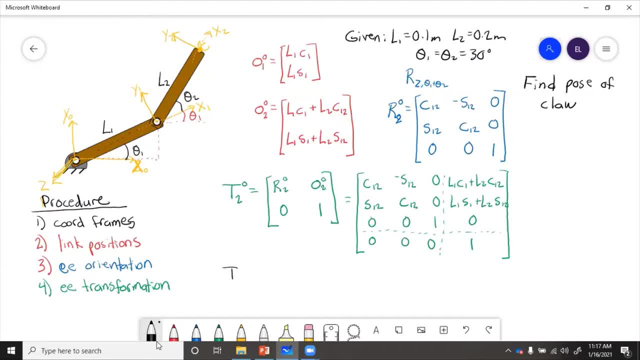 So t20 equals. let's see, we know that theta1 plus theta2 equals 60 degrees. So we just plug that into each of these: Cosine 60 minus sine 60, sine 60, cosine 60. So then we'll get, we plug those in 0.5, 0.866 minus 0.866, 0.5, 0, 0, 0, 0, 0, 0, 0, 1, 0..